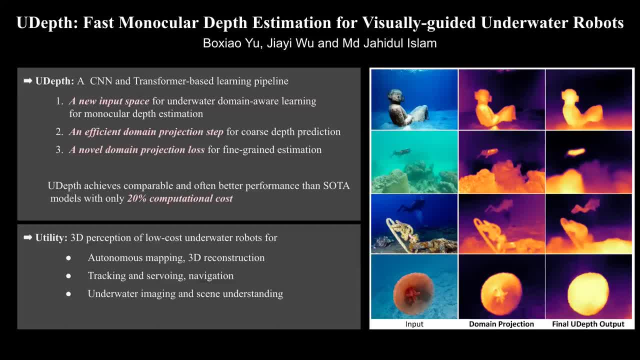 contributions in the UDEPs learning pipeline We adapt a new input space for underwater domain and variable learning. Then we design a computationally led projection step for core steps: prediction. We further devise domain projection laws to enforce attenuation constraints in the holistic learning process. Experimental results show that our model offers comparable. 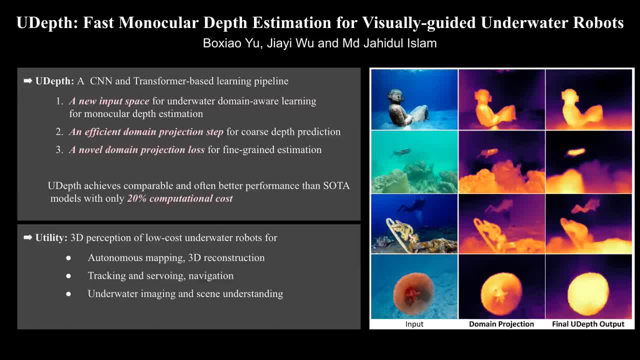 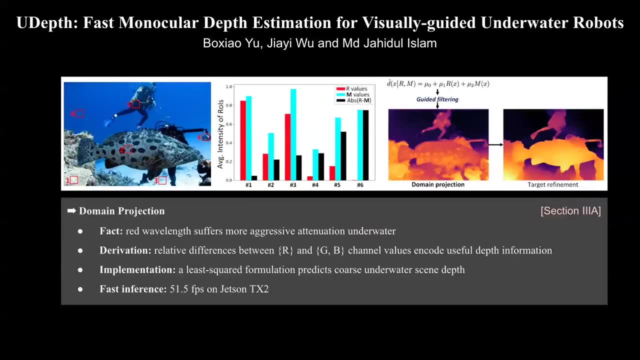 and often better depth estimation performance than social models, with only 20% computational cost. Our model can be used for onboard 3D perception by low-cost underwater robot for mapping 3D reconstruction in many important applications, As illustrated in this figure, we exploit the fact. 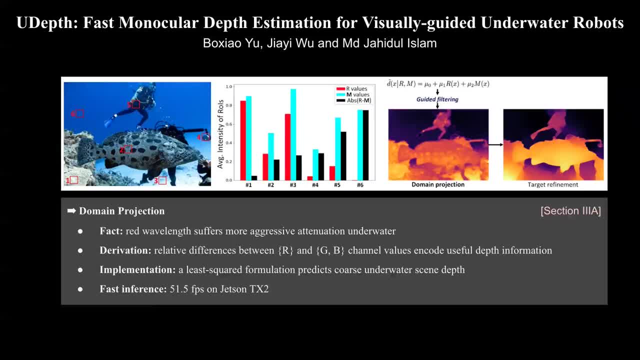 that red wavelength suffers more aggressive attenuation underwater, So the relative differences between R-channel and G-channel are not the same. The differences between R-channel and G-channel values can provide useful depth information for a given pixel. Based on this, we design a domain projection, step for pixel-wise. core steps: prediction by an efficient least-degree. 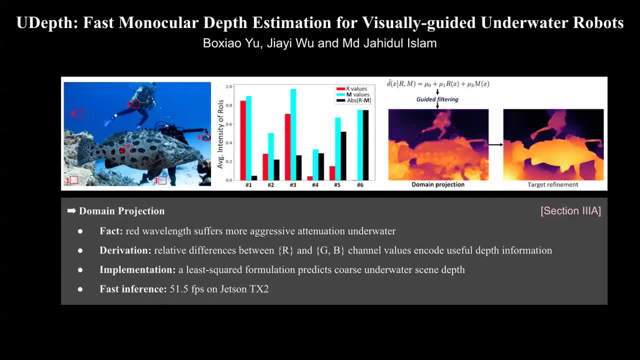 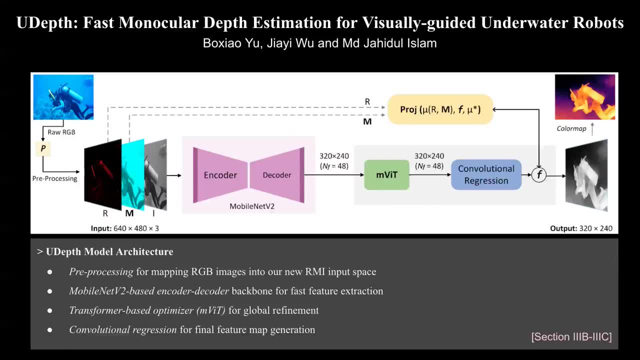 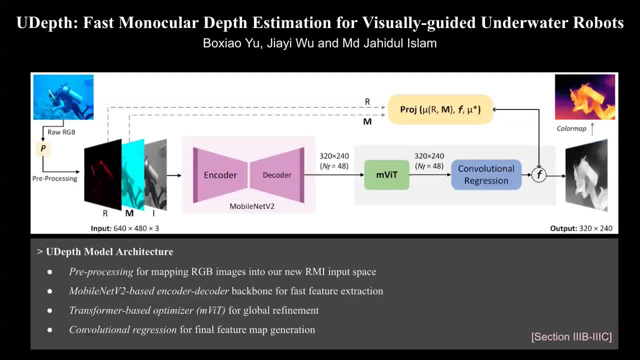 optimizer and followed by a convolutional regressor to generate the final single-channel depth prediction. The learning objective involves pixel-wise losses and a novel domain, projection loss. Please refer to the paper for more details. For the rest of the video, we will show qualitative results for UDEPs running on unseen nature: underwater images. 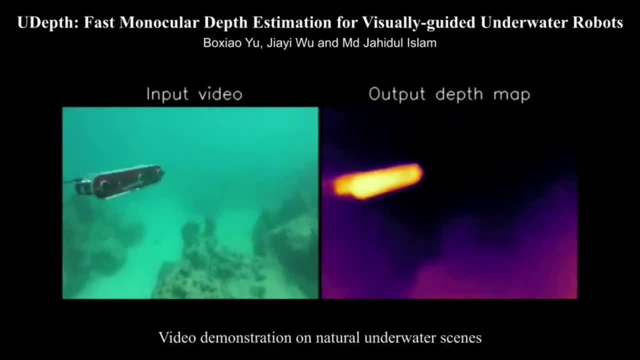 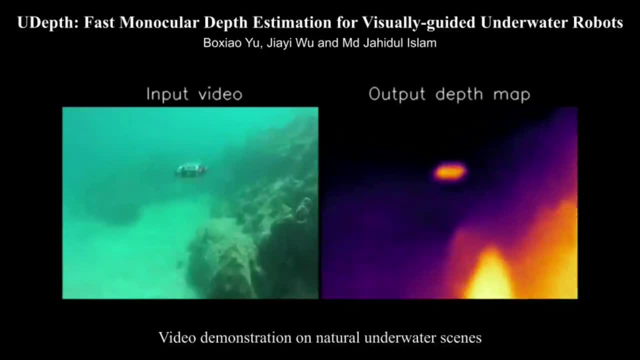 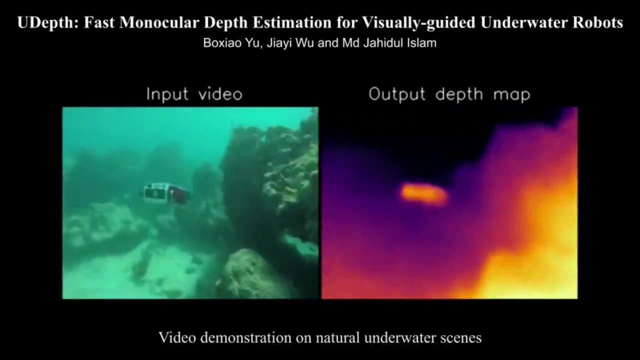 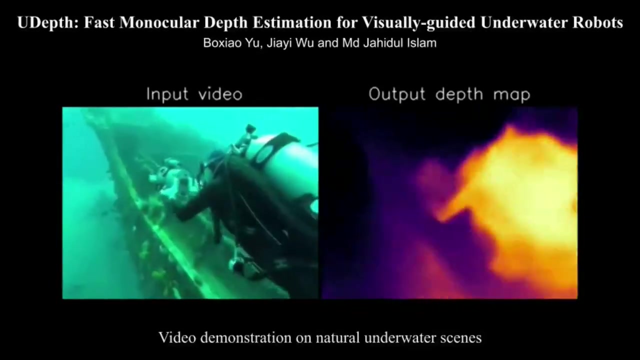 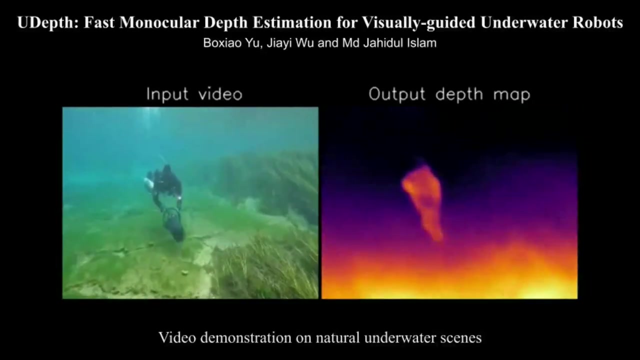 Thank you for watching. Thank you for watching.